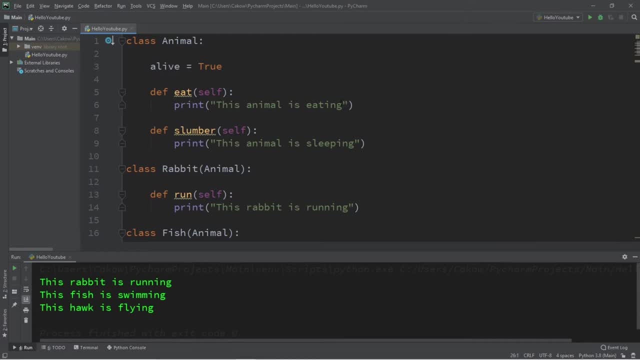 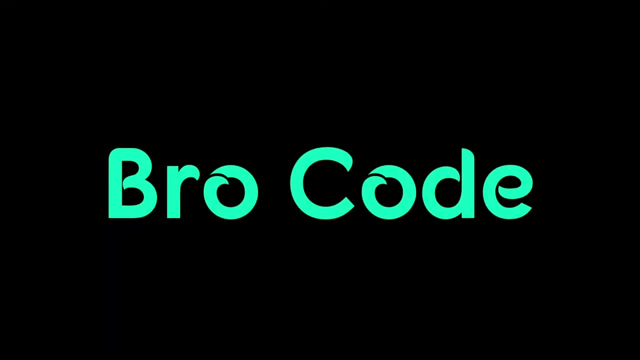 Hey, what's going on? everybody? It's your bro, Hope you're doing well And in this video I'm going to explain inheritance in Python. So sit back, relax and enjoy the show. If you find this video helpful, please remember to like, comment and subscribe Your support. 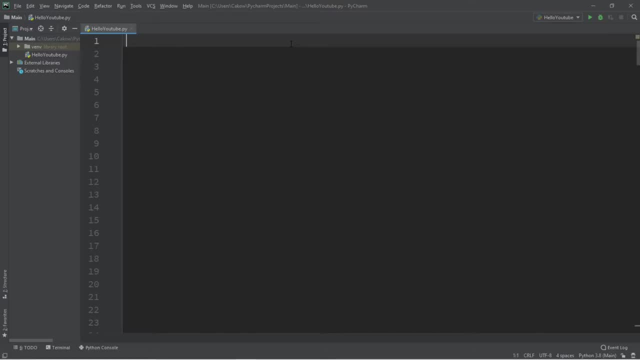 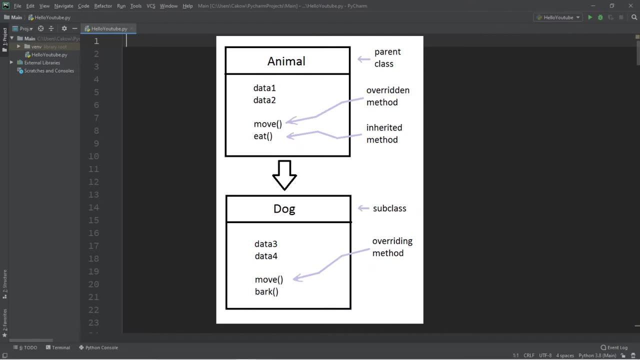 will help keep this channel running. Let's talk about inheritance. The term inherit means to receive, derive or be left with, and we can apply this concept to programming. Classes can inherit something, usually attributes and methods, from another class. These classes can form parent-child relationships where a child will receive everything that the 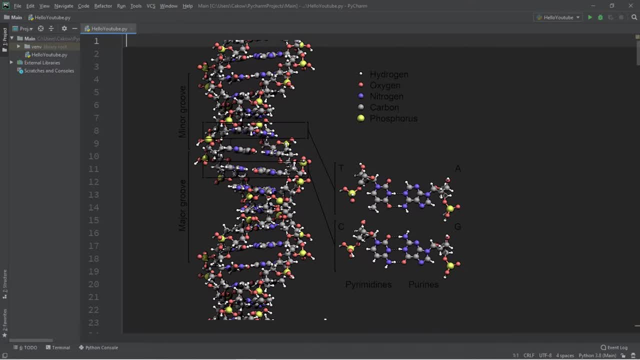 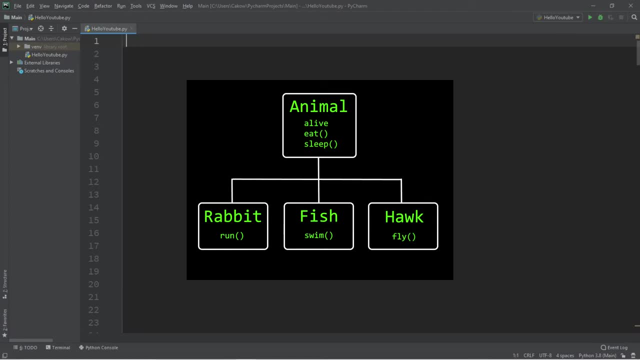 parent class has much like you- inherit genes from your parents, And classes can have children and give whatever they own to their children, And in today's video we'll be creating a parent class called Animal, And children of the Animal class will inherit the common attributes and methods. 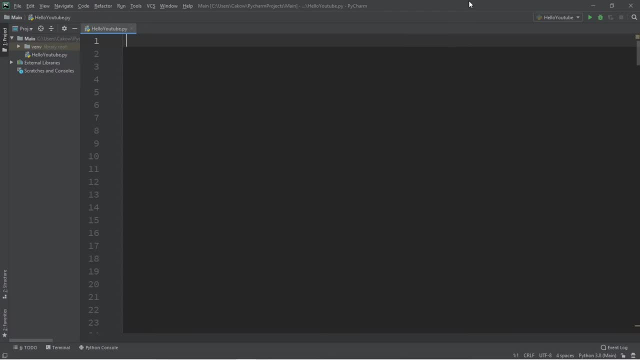 that all animals might have To kick off this video. I think what we'll do is keep all of our classes within the same file, just so that it's easier for us to read and understand. Let's begin by creating a parent-child relationship with the parent class. We're going to create a parent-child 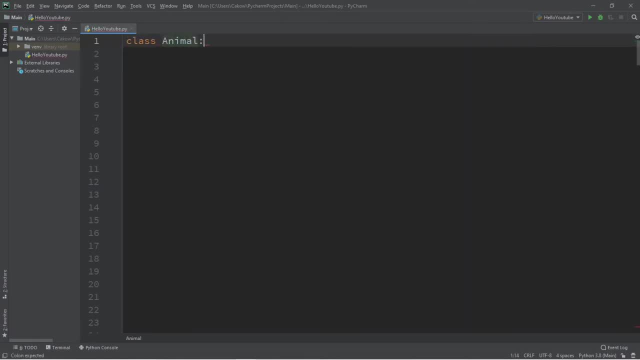 relationship by creating a class called Animal. So at the top type class, Animal, And what are some attributes and methods that all animals should have? Let's say we have a class variable called Alive and we'll set this to true: If you're an animal, you begin by being alive. 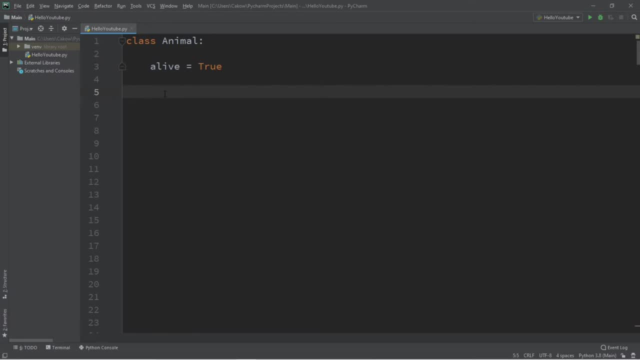 And what are some methods? How about an eat and sleep method? So let's define those DEF eat. What are we going to do when we call this method? Let's print something. Let's print: this animal is eating. Let's also create a sleep method: DEF sleep. 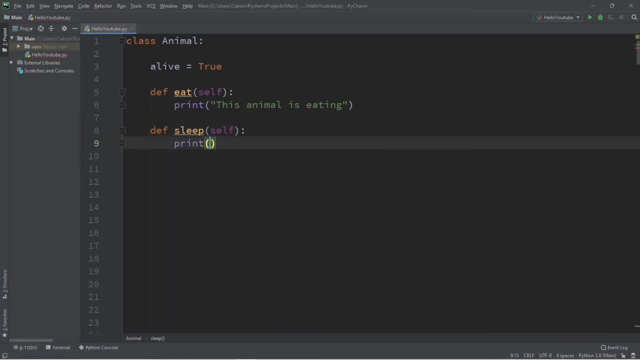 What are we going to do when we call this method? Let's print something as well: This animal is sleeping And we now have our Animal class. Now let's create separate classes for specific types of animals. Let's say, a class for rabbit, a fish and a hawk. 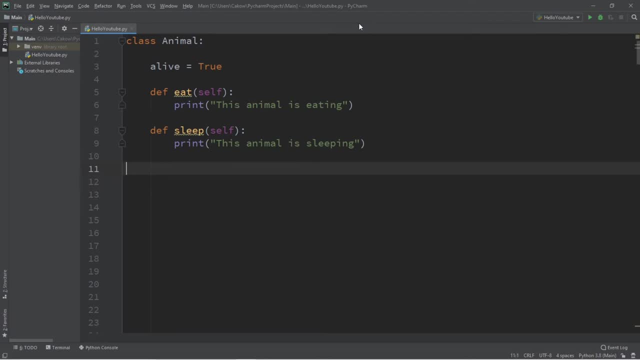 so we can make objects of those classes. So let's begin with a rabbit class Class rabbit. Now to use inheritance with the class that you intend to be the child class, after the class name add a set of parentheses And then pass in the name of the parent class. In this case it's going to be animal. 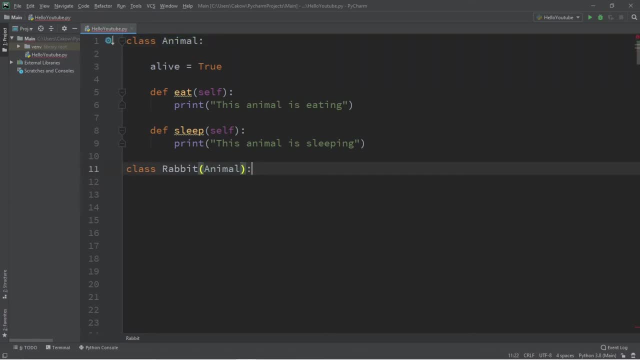 so we will add that to the parentheses. So now rabbit is the child class and animal is the parent class. So the child class is going to inherit everything that the animal class has. So for the time being I'm going to type pass, So this rabbit class will. 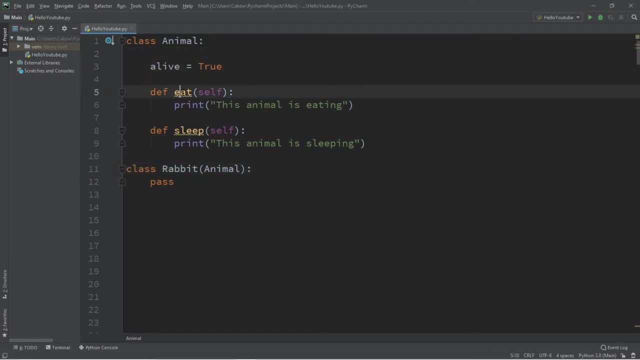 have access to a class variable called Alive and an eat and sleep method. So let's define a fish and hawk class And I'm just going to copy what I have here and just change rabbit to fish and then do so again and change rabbit to hawk. This is our family tree Animal. 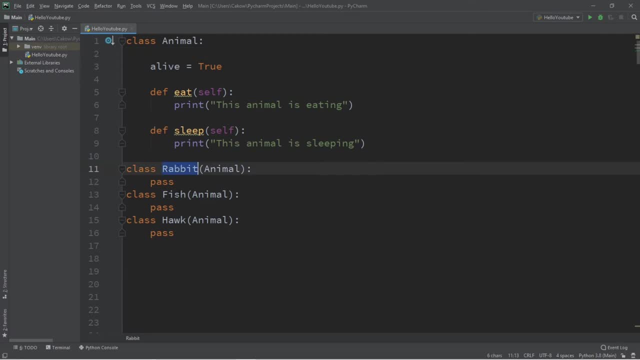 is the parent class and it has three children: a rabbit class, a fish class and a hawk class. And for the time being we're just going to write pass as a placeholder. So I bet we can create objects from these classes. So let's do so, Let's say we have. 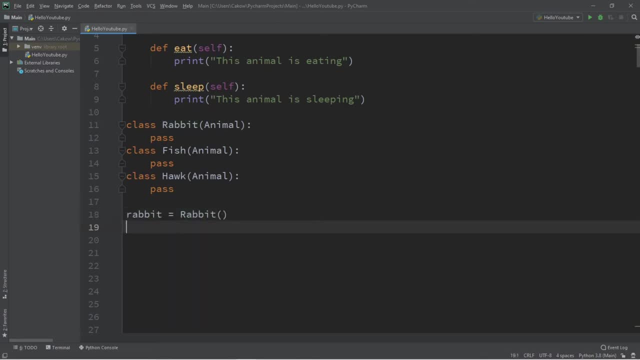 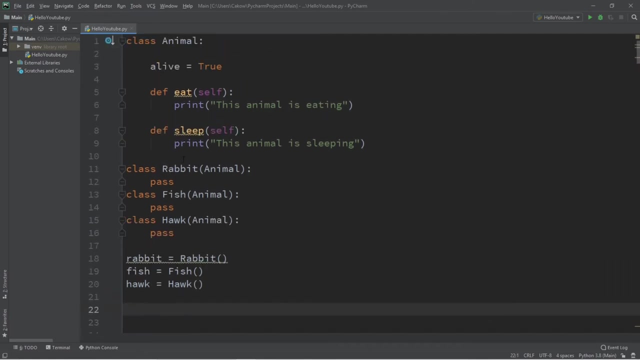 an object called rabbit. Rabbit equals rabbit. Let's do the same thing for fish and hawk. All right, we now have three objects- Rabbit, fish and hawk- And let's take a look at their class variables. I bet they have an alive variable. Let's check that. So I would like to 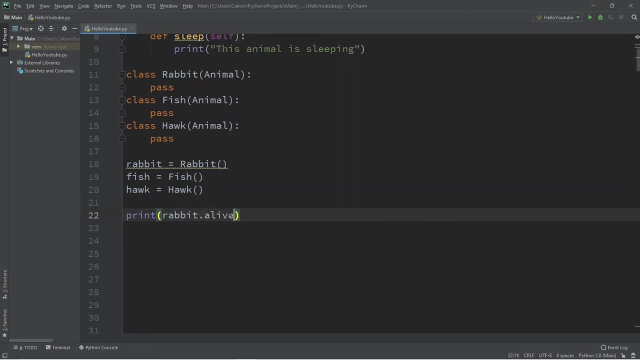 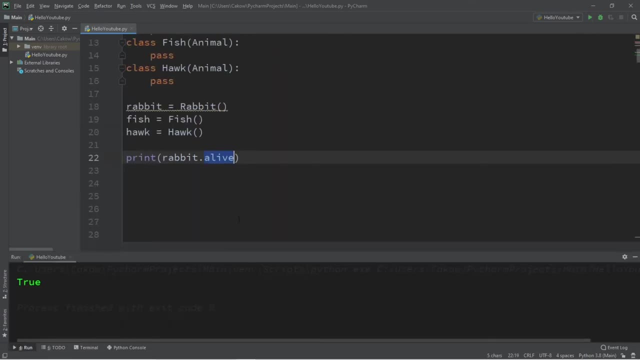 print rabbit dot. oh, would you look at that? This rabbit class has a class variable called ALIVE, even though there's nothing within this class. Well, that's because we used inheritance, So each of these three children classes inherit everything from their parents, All of these attributes and 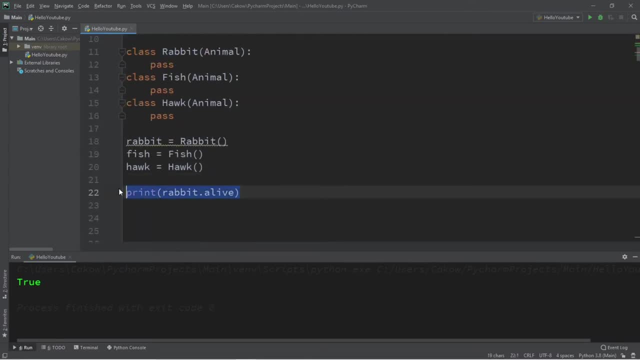 methods. So I bet we can create objects. And that's the next step. Let's just cut this out, So we have this class as an object. I would like to take this class as now. Now I have three classes. I bet they have eat and sleep functions as well, so let's check that. 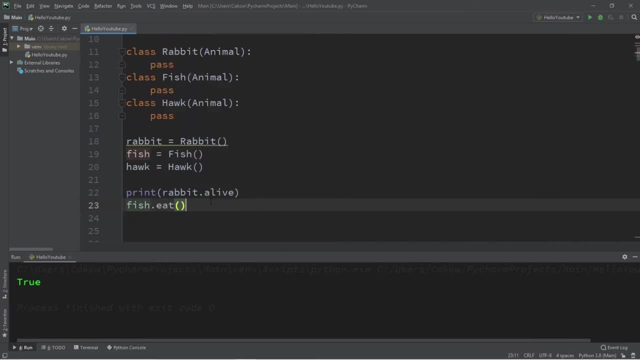 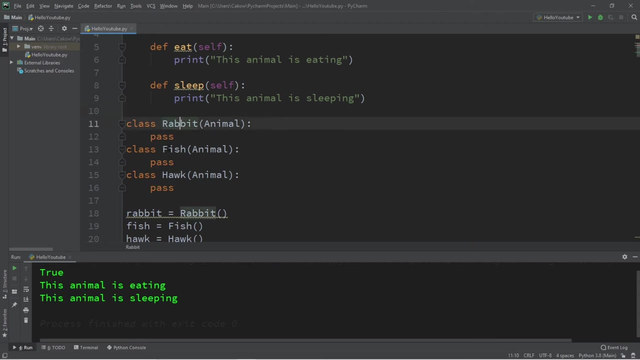 With fish. let's have fish use its eat method and hawk will use its sleep method- hawksleep. So the rabbit is alive, the fish is eating and the hawk is sleeping. Now, even though we have nothing written within each of these specific types of animal classes, 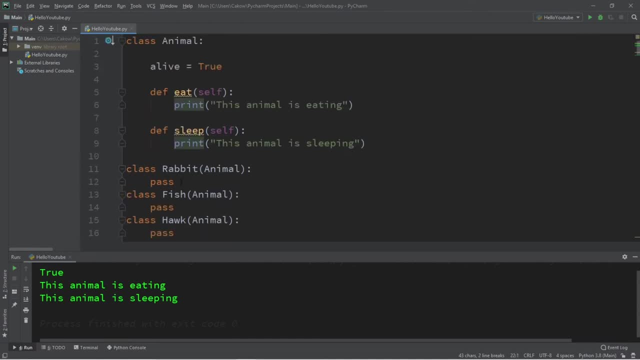 all of these animals have access to these attributes and methods because of inheritance, And another benefit of inheritance is that we don't need to keep on copying and pasting this code. For example, let's say we were not using inheritance, so we would not need an animal class. 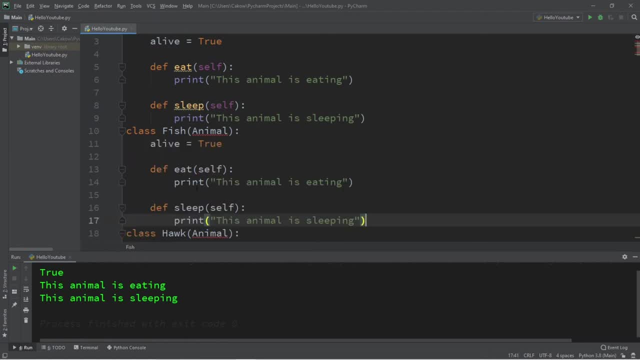 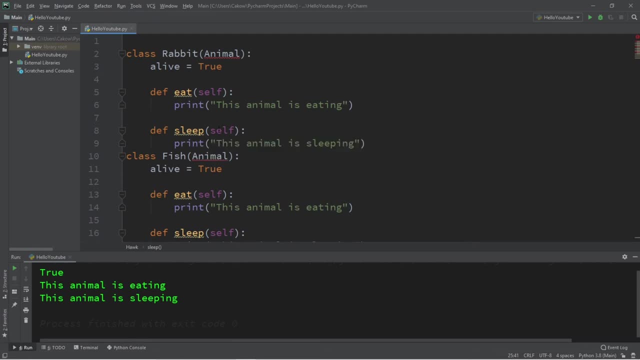 We could write our code this way, where we would just copy and paste everything underneath each of our classes. So what if we need to make a change to one of these methods, As in your boss says: you know what? let's change. sleep to slumber, okay. 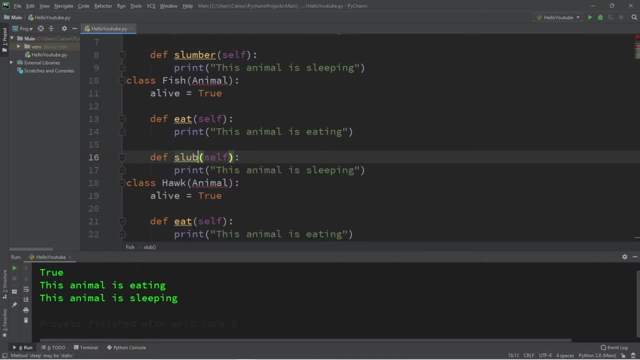 Well, we would have to go to each of these classes and make the change manually. It's not too bad if you have like three or four classes, But what if you have hundreds? That's going to take a lot of effort. 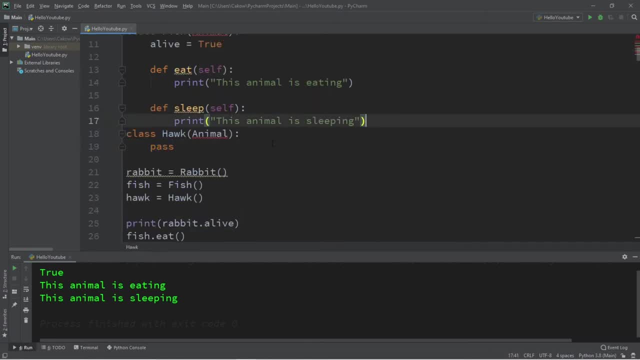 So wouldn't it be nice if we just list everything that each of these classes has in common and then have all of these classes inherit from one common class, And then if you need to make any changes, you can do so just within this class? 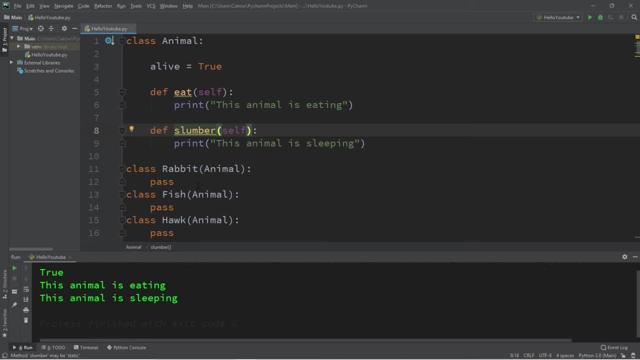 And this change will apply to all of the different child classes. So that's another benefit of inheritance, And not only does it make any changes easier, but each class can have their own unique attributes and methods as well, Along with the attributes and methods that they inherit from their parents. 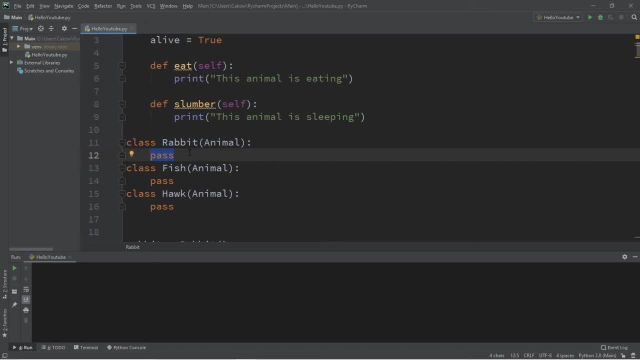 So for rabbit, fish and hawk, let's have each of these classes have their own unique method as well. So for rabbit, let's define a run method. If you're a rabbit, then you can run, So let's print this: rabbit is running. 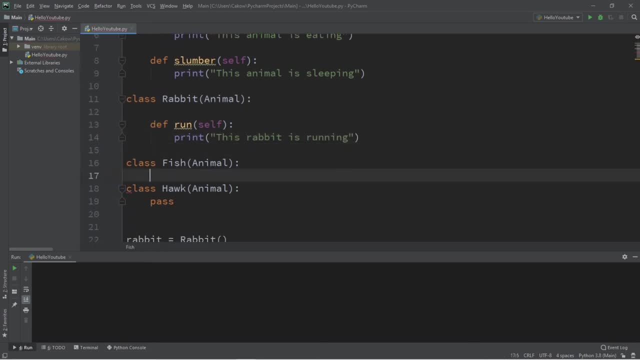 And I'm just going to fix some of the spacing here. Alright, if you're a fish, then you can swim. Def, swim. Let's print: This fish is swimming. And lastly, we have hawk. If you're a hawk, then you can fly. 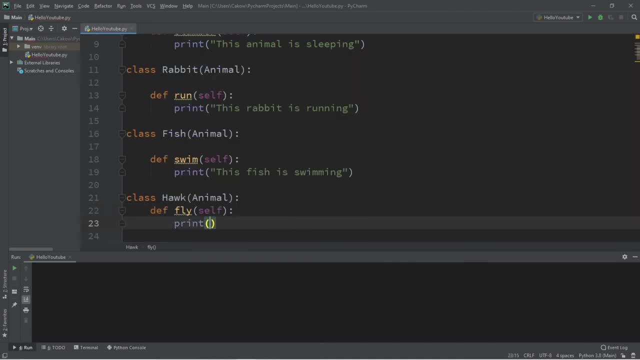 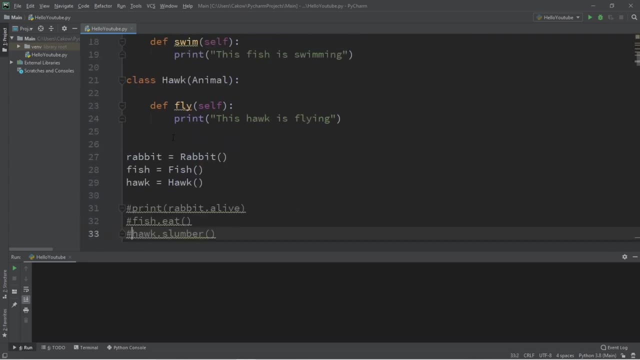 Def fly, Let's print. This hawk is flying. Like I said before, not only do these specific types of animals have access to all of the attributes and methods that they inherit from their parents, but they can have their own attributes and methods as well. 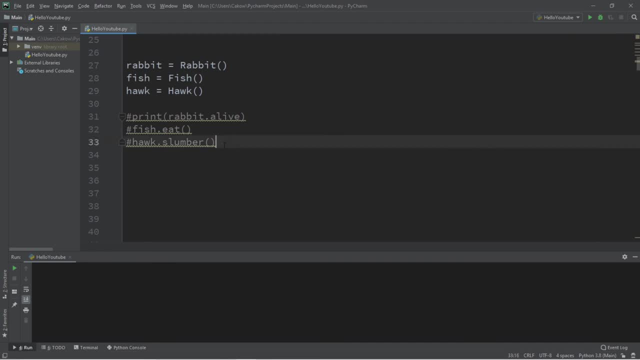 So let's test some of these methods. So we have our rabbit, fish and hawk objects. Let's have rabbit use its run method, Fish will use its swim method And hawk will use its fly method. And here we go: This rabbit is running, this fish is swimming and this hawk is flying.